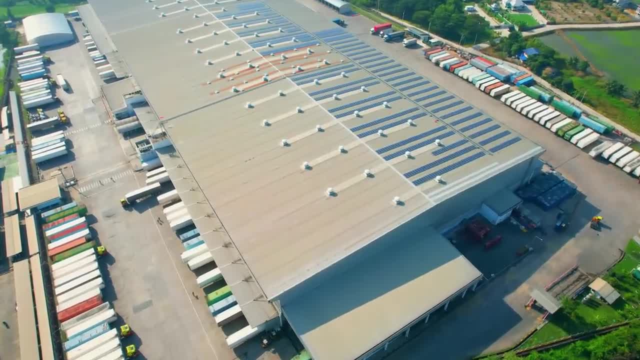 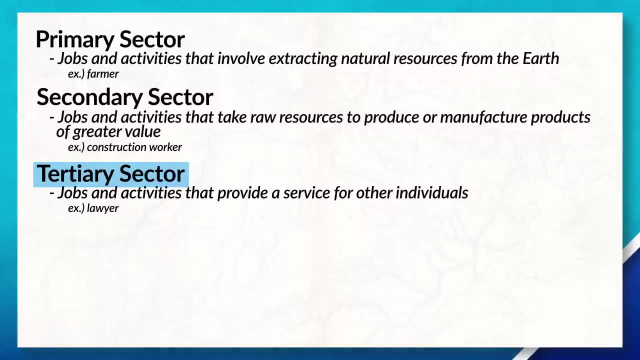 that supports the shipping of resources and final goods. Now the next sector of the economy is the tertiary sector. Here, jobs and activities are based around providing services for people. Jobs and activities in this sector are often located near jobs in the primary sector to help reduce the cost of transporting raw resources. 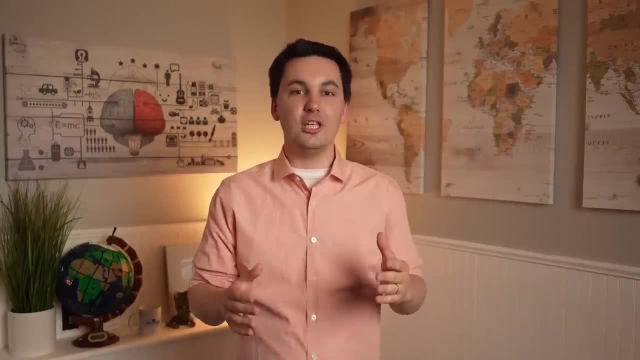 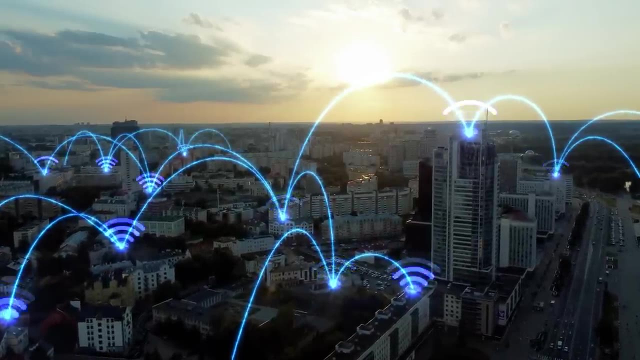 are often located near consumers and are where there is a need for that specific service. However, even this is starting to change thanks to advancements in technology, as more services are being provided over the internet to different geographic areas, such as the case with this video. 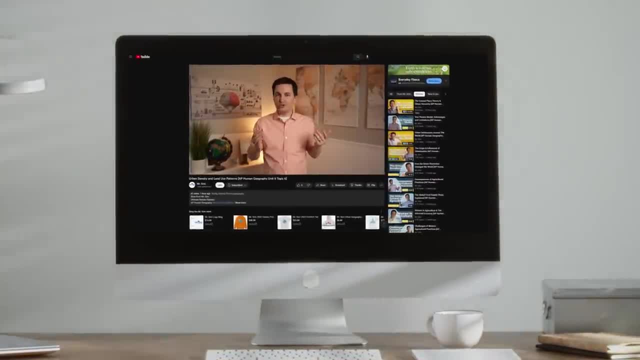 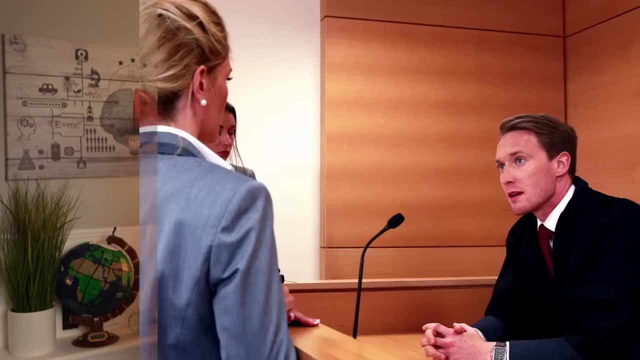 I'm helping you review for AP Human Geography and there's a pretty good chance that we don't even live in the same state or maybe even the same country. Examples of jobs in the tertiary sector would be lawyers, doctors, servers, Uber drivers. 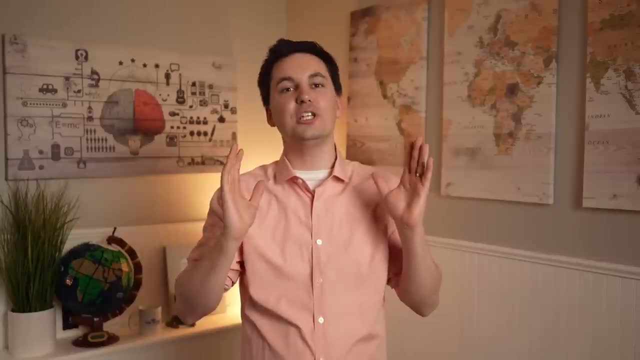 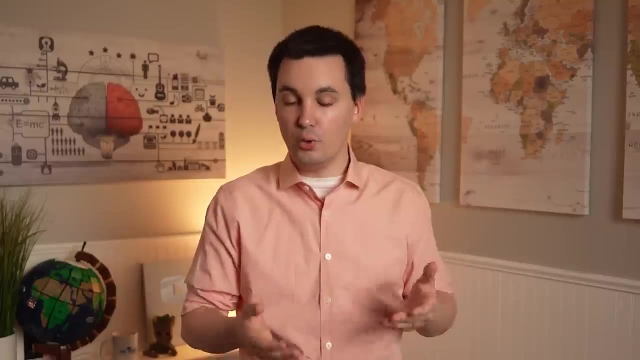 real estate agents, door dash drivers- and that's only naming a few. We can see that as countries continue to develop economically, it's common to see more and more jobs move out of the primary and secondary sector and move into the tertiary sector of the economy. 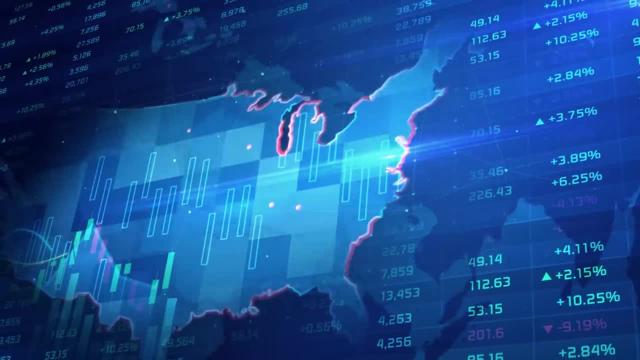 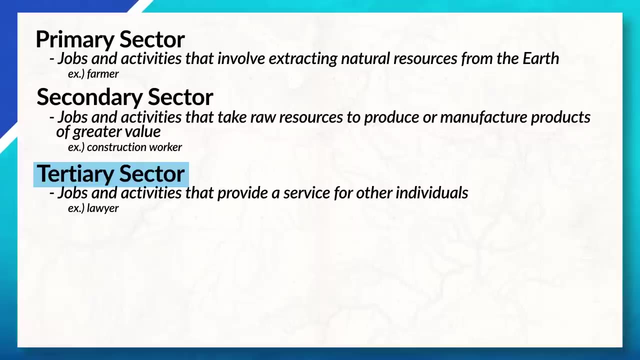 In fact, today the majority of the United States' economy is located in the tertiary sector. Now, the last two sectors of the economy are actually subsectors of the tertiary sector, The first one being the quaternary sector, which consists of jobs. 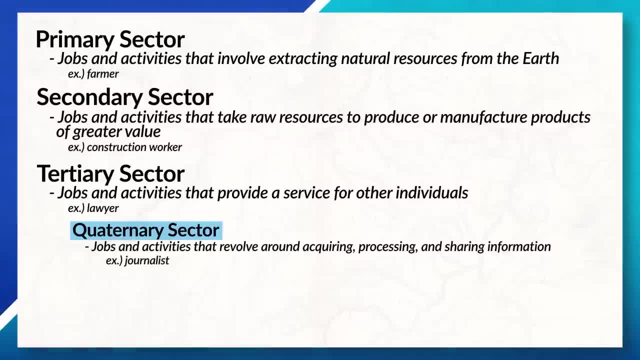 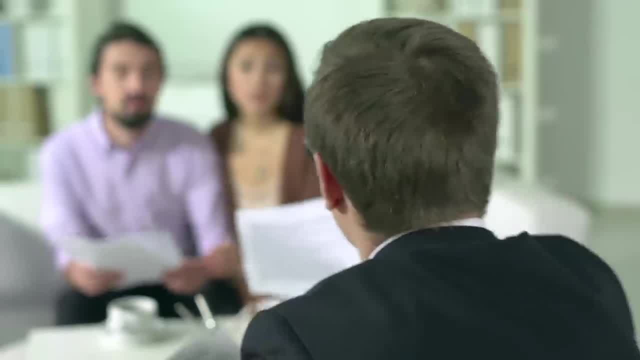 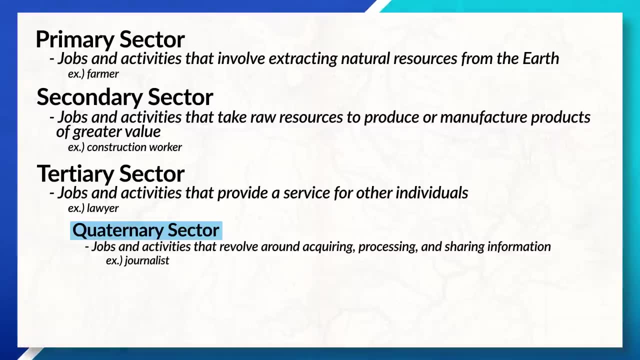 and activities that are all about acquiring, processing and sharing information. Located in this sector would be teachers, professors, journalists, people in finance, insurance or other industries that are centered around information collection, processing and distribution. Lastly, there's the quinary sector. 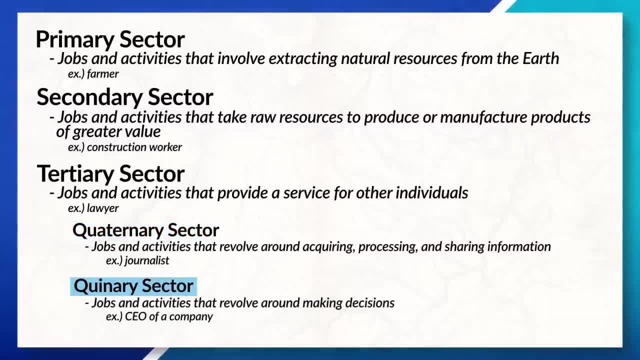 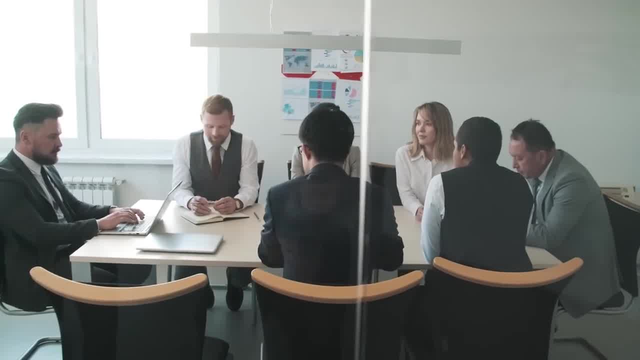 which consists of jobs and activities that revolve around making decisions: For example, politicians of a country, such as a senator or the president of the country, or executives of a company or the CEO of a company, such as Steve Jobs or Elon Musk. 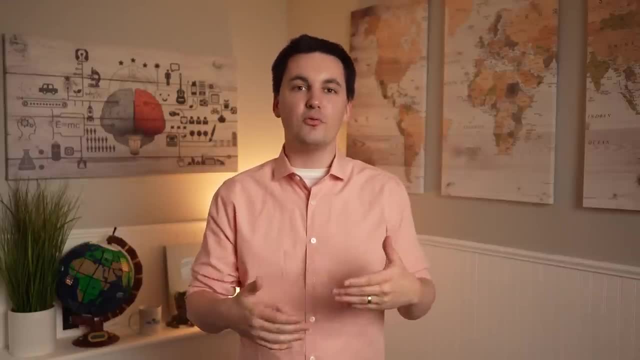 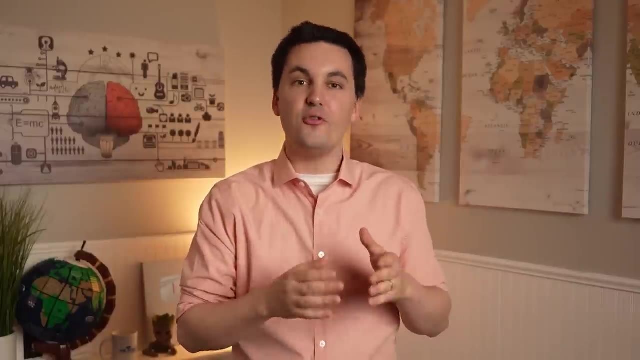 knows that both the quaternary sector and the quinary sector are still providing services. That's why they're part of the tertiary sector. However, these sectors are more specialized and are focused around specific aspects of what the service is, ultimately setting them apart from other jobs. 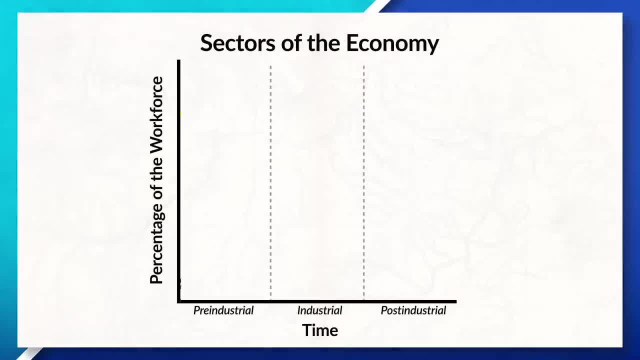 in the tertiary sector. Now, as countries develop economically, we tend to see economic transformations occur. For example, countries that have not yet industrialized. they'll often have more jobs than others. and they'll have more jobs than others In the quaternary sector. 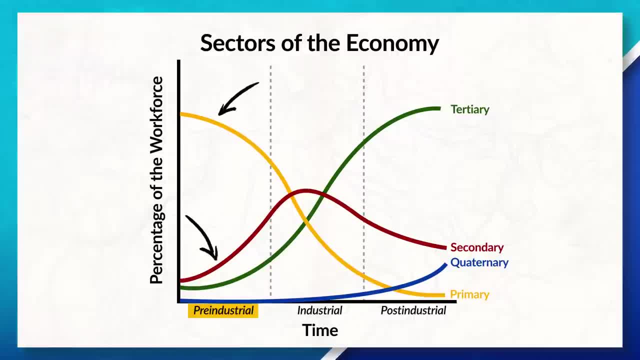 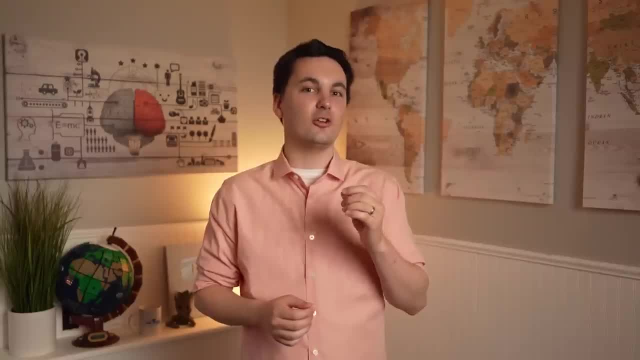 we have jobs located in the primary sector, with only a few jobs in the secondary and tertiary sector. Over time, as economic development occurs, we start to see the rise of jobs in the secondary sector and eventually, the tertiary Jobs in the secondary sector start to become more dominant. 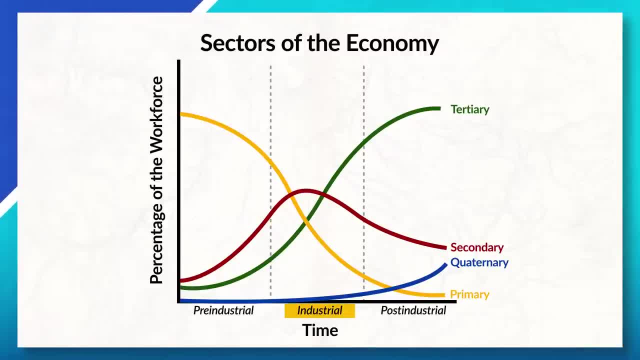 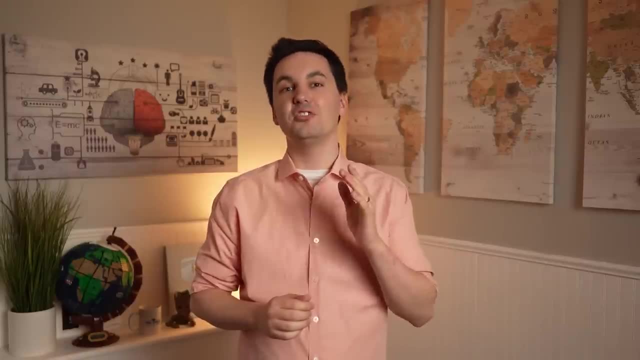 once the economy becomes industrialized. Here we can see jobs in the primary sector drastically start to decrease as more jobs open up in the secondary sector and also the tertiary. Now, as development continues, we will eventually see a shift from an industrial society to a post-industrial society. 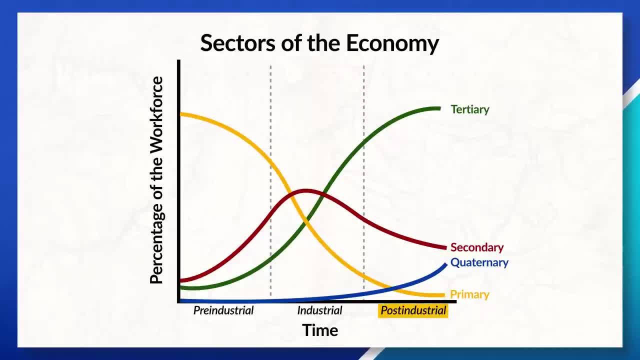 This is when deindustrialization often occurs and jobs in the secondary sector start to decline, while at the same time jobs in the tertiary sector start to expand. Here, the economy is becoming more focused around service jobs and less on manufacturing. 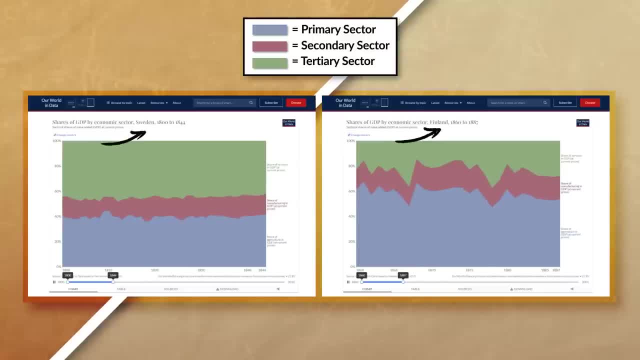 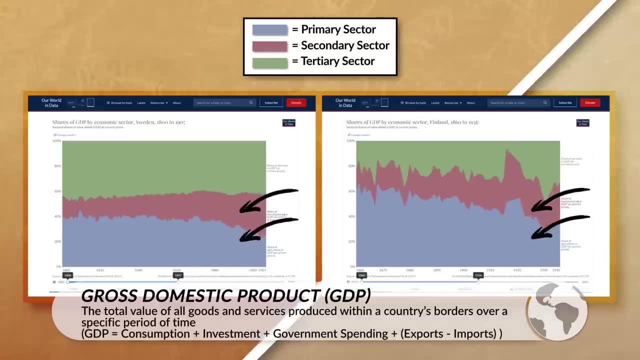 You can see this trend here. when looking at Sweden and Finland, Notice how both countries originally had a fair amount of their GDP located in the primary sector and the secondary sector, but over time each of those sectors declined, with the decline first starting in the primary sector. 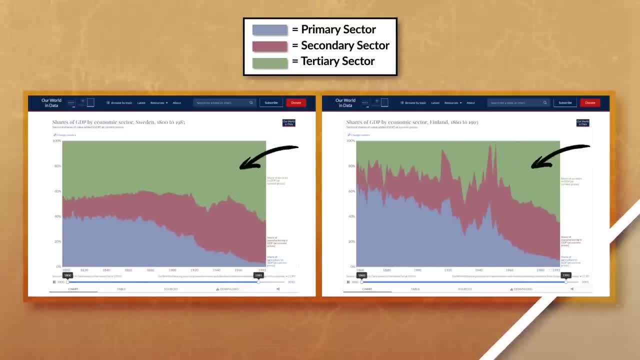 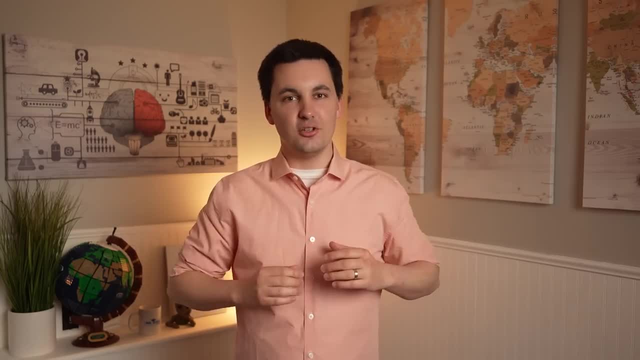 and then the secondary sector, while at the same time the tertiary sector continued to account for more and more of the GDP in the country. So we can see that countries that are less economically developed will tend to have more jobs in areas such as agriculture. 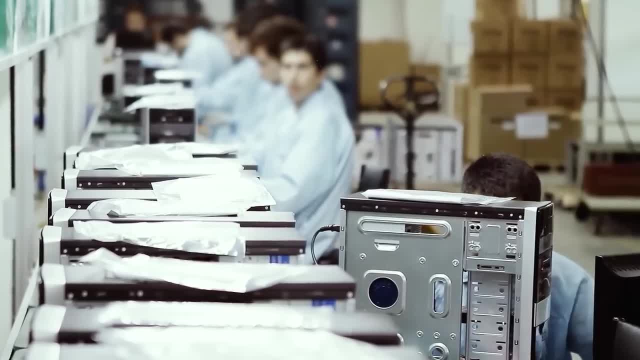 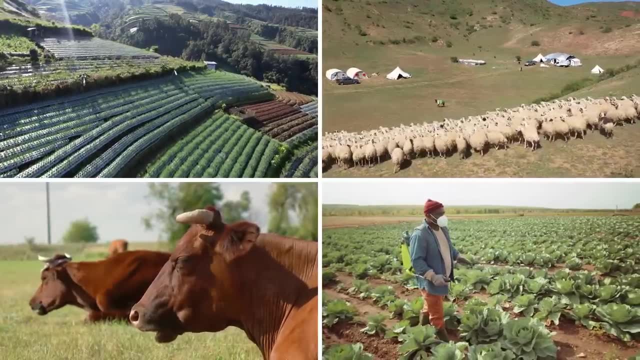 and countries that continue to have an emerging economy as they experience industrialization will start to see more jobs open up in manufacturing, All of which connects back to our agriculture unit, where we looked at food production around the world. We will continue to explore these different development trends further. 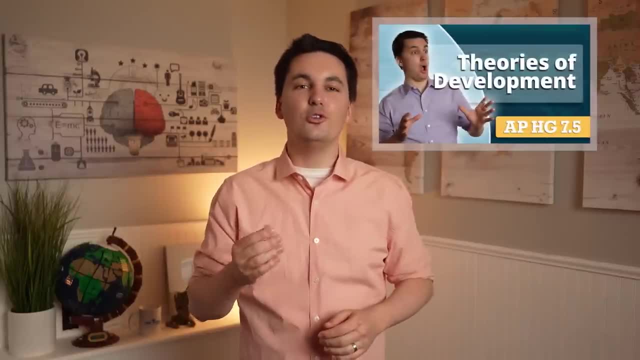 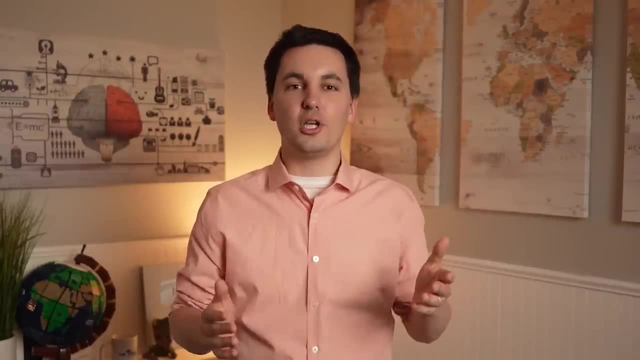 when we talk about Rostow's stages of economic growth in our Unit 7, Topic 5 video. Now, since we've spent some time talking about the different economic sectors, we also need to look at how we can classify countries based on their economic development. 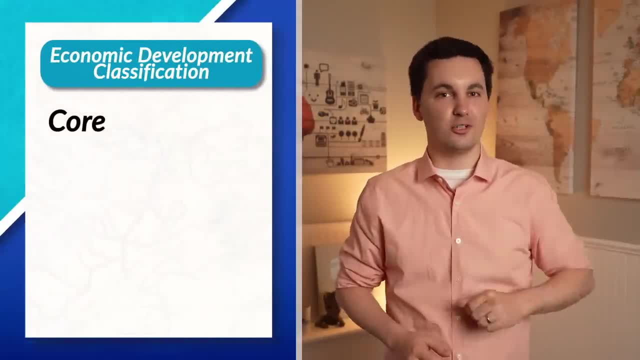 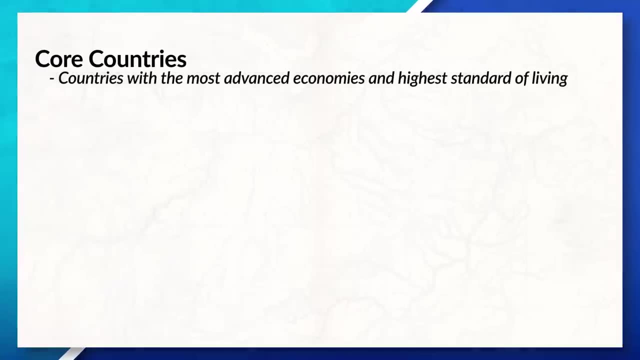 Throughout this course, we will continue to reference countries as core countries, semi-periphery countries and periphery countries. core countries tend to have the most advanced economies, typically have a higher standard of living and have more of their jobs located in the tertiary sector. 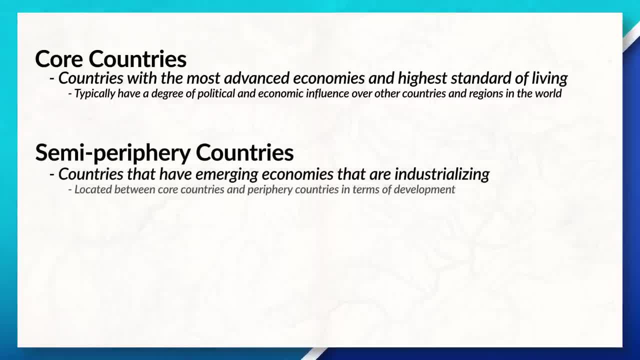 Semi-periphery countries are countries that have an emerging economy, are experiencing an increase in their standard of living and have many jobs in the country located in the secondary sector, as more industrialization continues to occur. Lastly, there's periphery countries, which tend to have a lower standard of living. 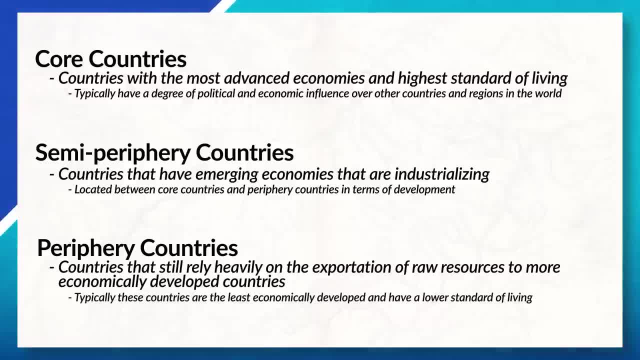 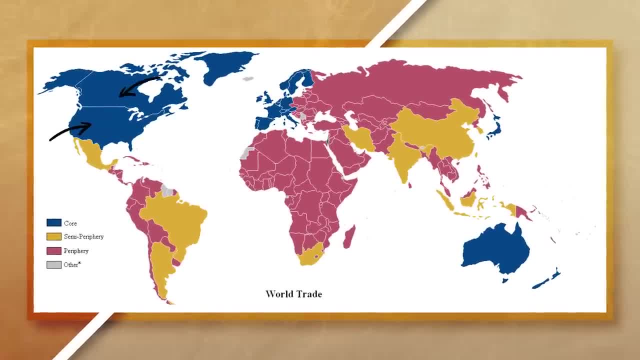 since industrialization has not yet happened yet, causing many of the jobs in the economy to be located in the primary sector. When looking at the world today, we can see that the United States, Canada and many European countries are considered core countries. 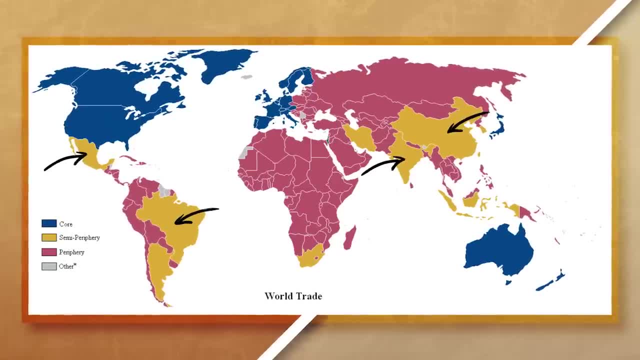 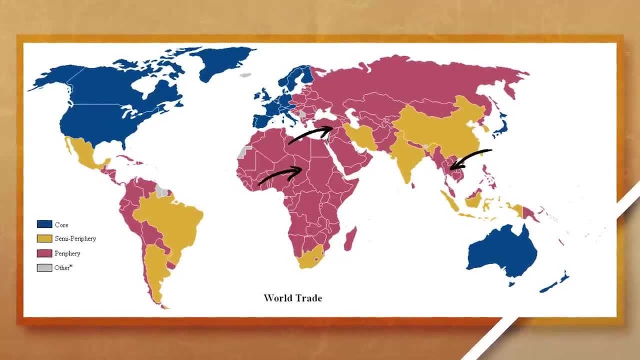 while countries like China, Brazil, Mexico and India would be examples of semi-periphery countries, And we can see that many countries in Africa, the Middle East and parts of Asia would be example of periphery countries. Now, if we take our understanding of economic sectors, 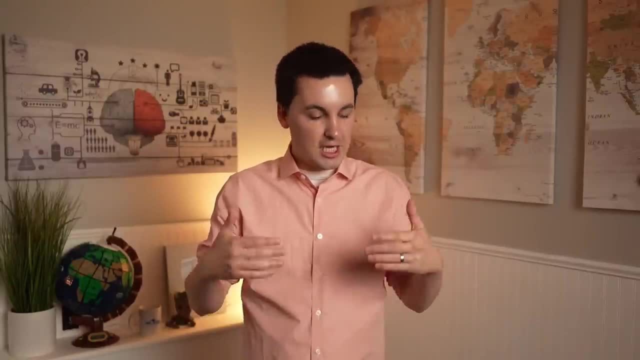 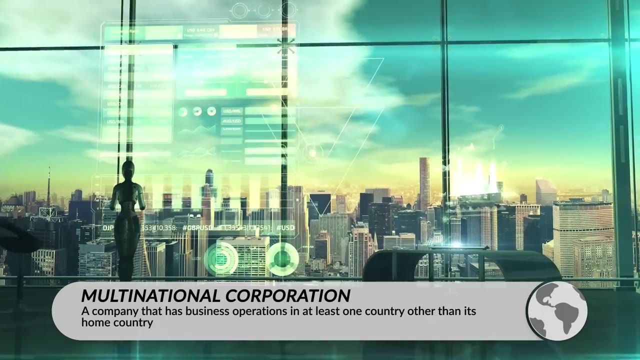 and development and look at global production, we can gain even more insight into global patterns. We can see that many multinational corporations often locate their production facilities in periphery and semi-periphery countries in order to help reduce their costs and take advantage of cheaper labor. 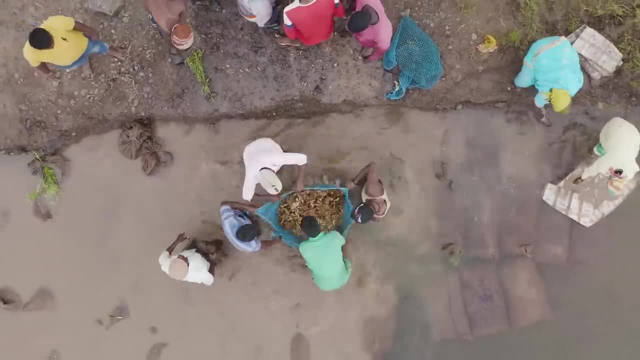 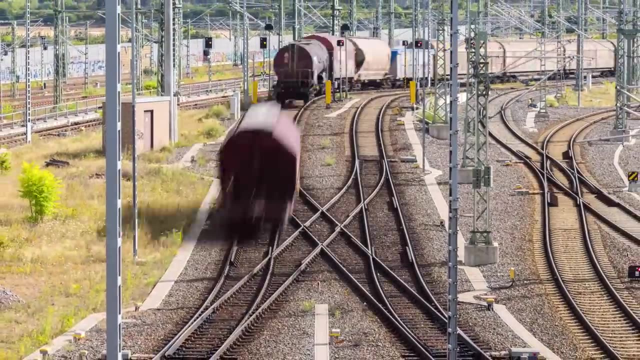 and more loose regulations in the area. This trend has continued over the years, partially due to advancements in transportation, which now make it easier than ever to transport raw resources and finished products around the world, allowing for the creation of complex supply chains to form. 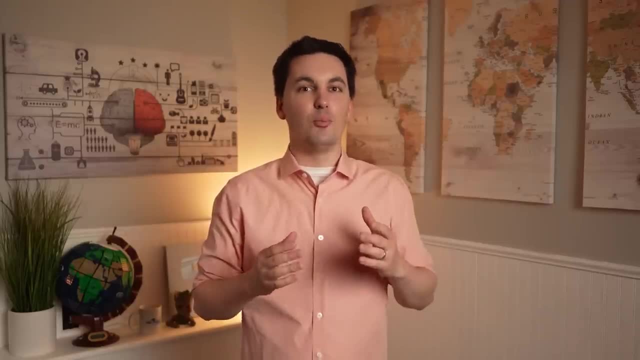 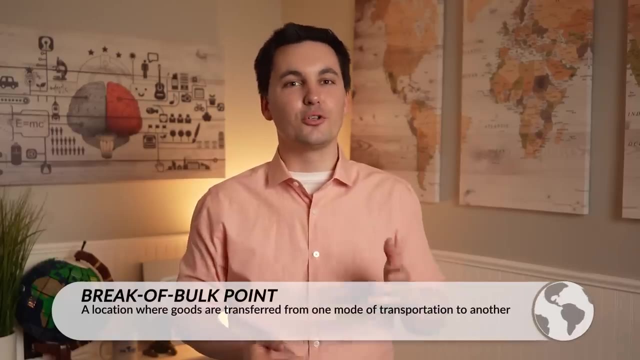 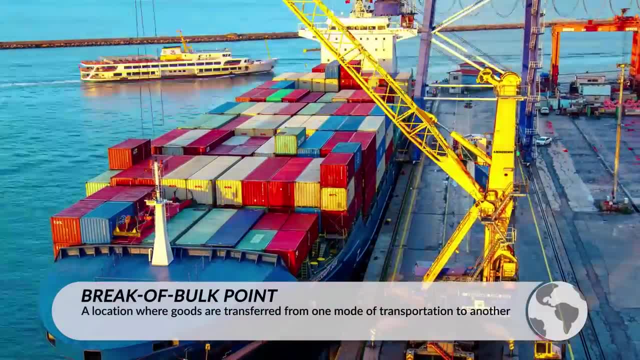 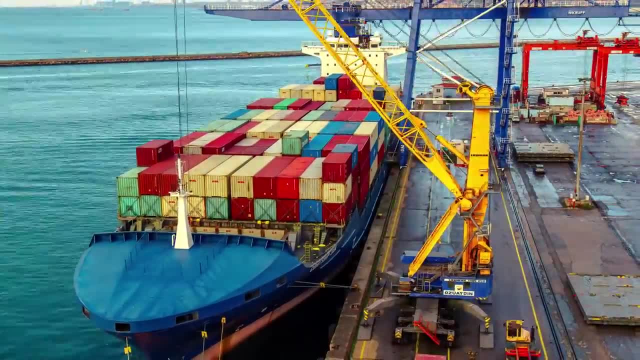 from one mode of transportation to another. For example, ports are a break of bulk point where cargo ships unload the goods they are carrying and place those goods on different trucks or trains. The goods are then transported inland to get to a distribution center or to one of the different places. in which the goods will be sold. Companies that participate in the global economy often are able to reduce the cost of production, produce more goods and lower prices for consumers, All of which sounds good, but at the same time, these patterns have also led to unequal economic development. 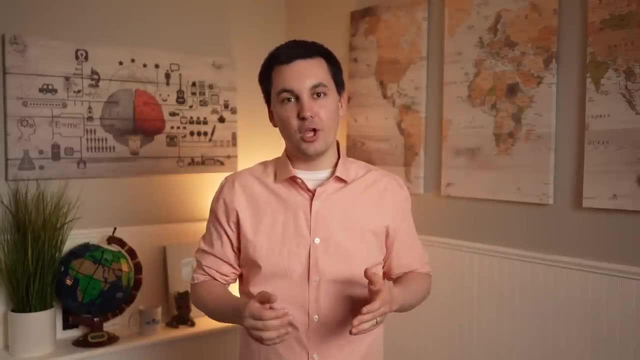 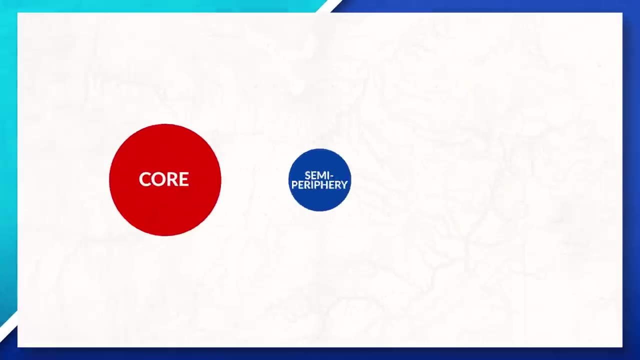 around the world, As countries that are in the periphery and semi-periphery often see disproportionately less economic gains from this global trade compared to the core countries. We will explore these global relationships more when we go into Wallerstein's world system theory later in this unit. 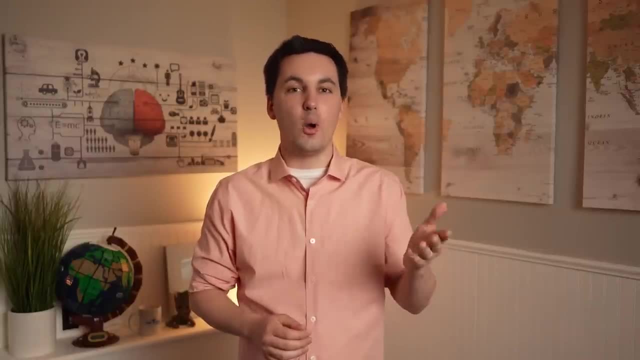 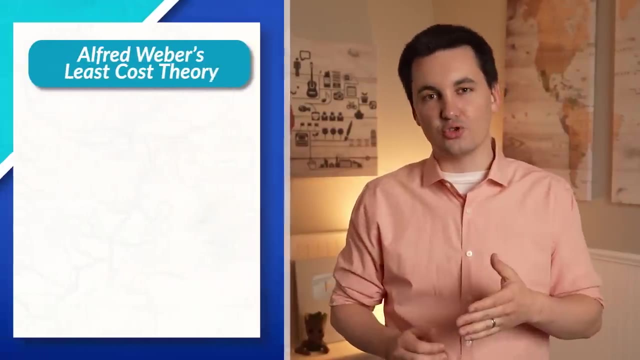 Now, since we're on the topic of production, we also need to review Alfred Weber's Lease Cost Theory, also known as the Theory of Industrial Location. The theory looks at how the location of an industry is influenced by three main factors: Transportation costs, labor costs and agglomeration. 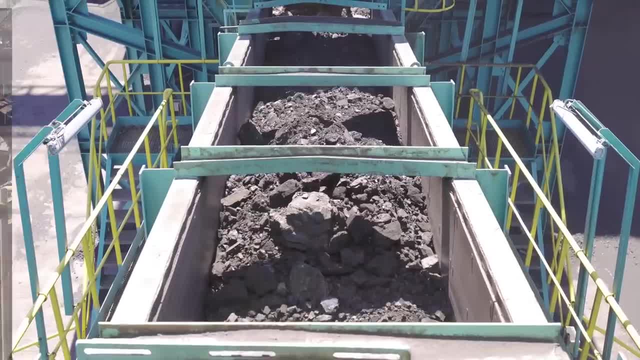 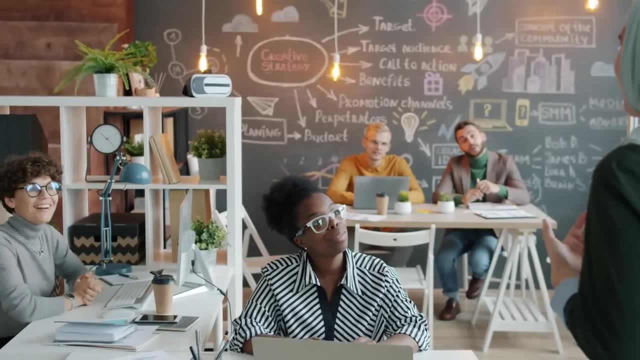 Transportation costs are shipping costs connected to the moving of resources and materials for producing a good and shipping the final product to the market. Labor costs, on the other hand, are costs that come from workers producing the product itself. Lastly, agglomeration is the clustering. 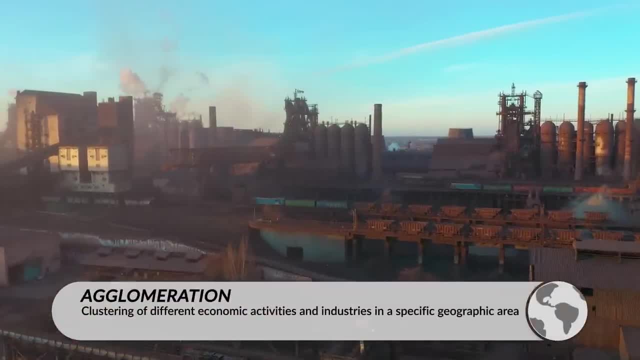 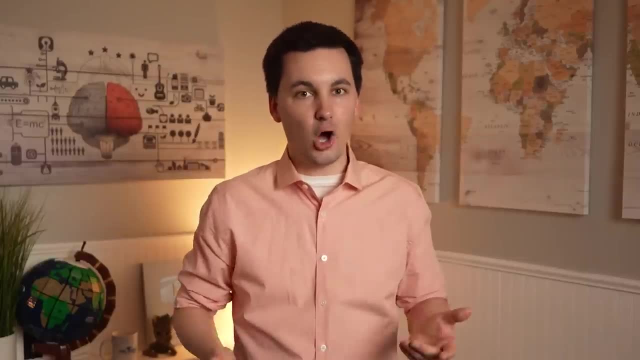 of different economic activities and industries in a specific geographic area, which might sound weird at first, but there's a reason why this happens. It allows businesses to reduce their overall costs by taking advantage of larger labor forces benefiting from the existing infrastructure in an area. 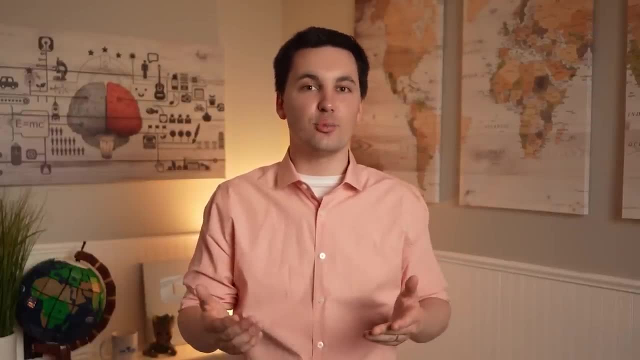 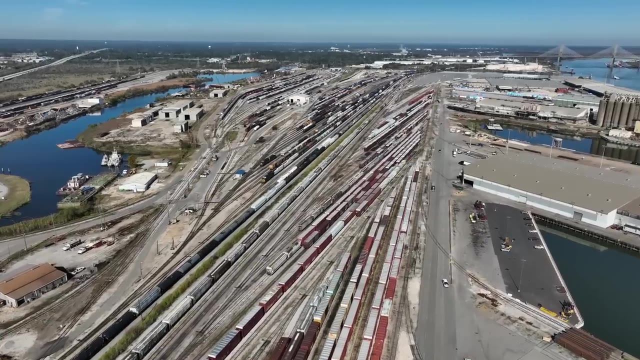 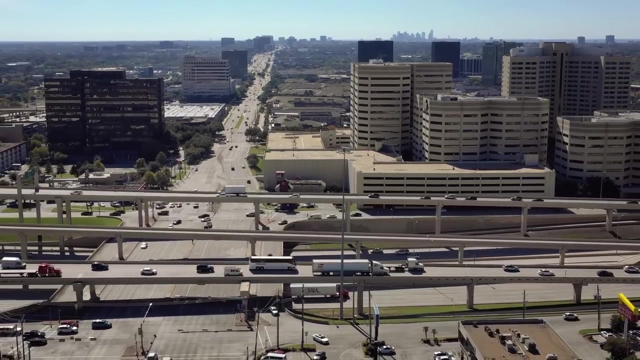 and by allowing businesses to use the different services and knowledge base in a specific area. For example, we can see that many distribution centers are located near major interstates, airports and ports. This allows them to use the pre-existing infrastructure in the area instead of having to build it themselves. 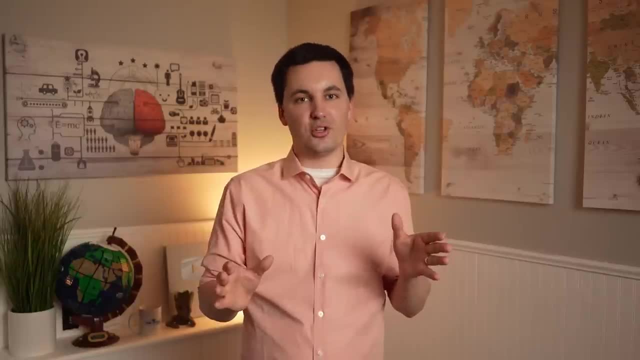 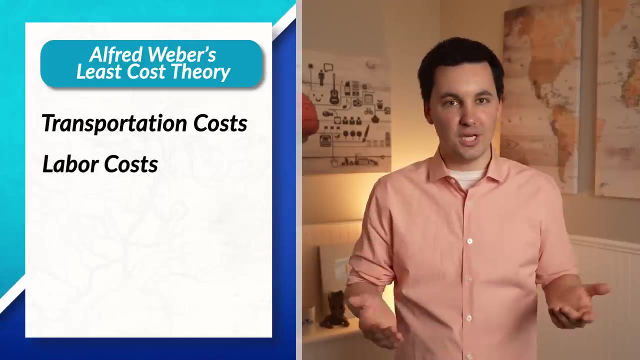 which reduces their overall costs of production. Now Weber's Least Cost Theory states that the location of production should be located in an area where transportation and labor costs are minimized and the economic benefits of agglomeration are maximized. For simplicity's sake, let's say we are looking 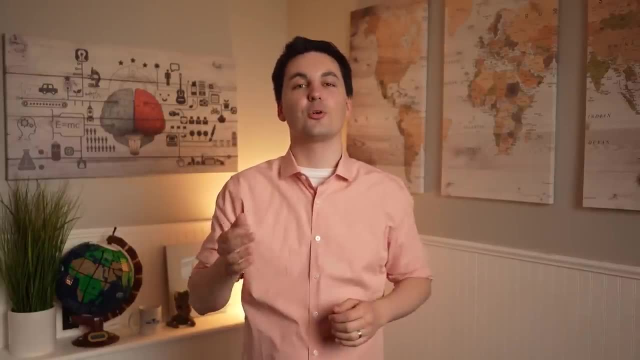 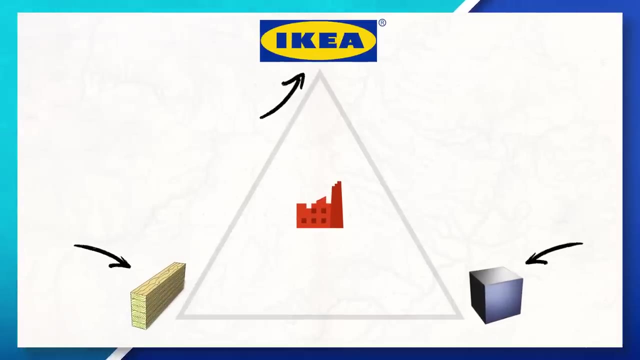 at producing a product that only needs two resources for the production of the final product. If we look at Weber's theory, we can see that we have different resources, a market and, inside the region, the optimal location for the production of our product. 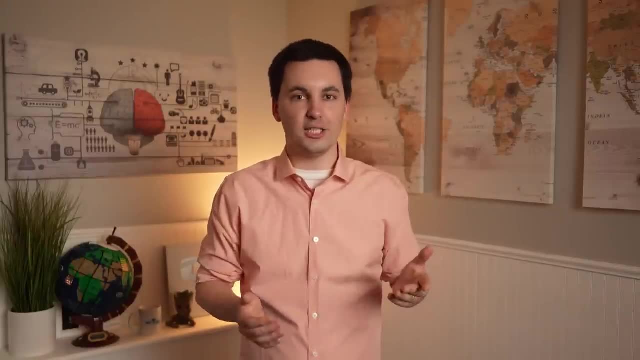 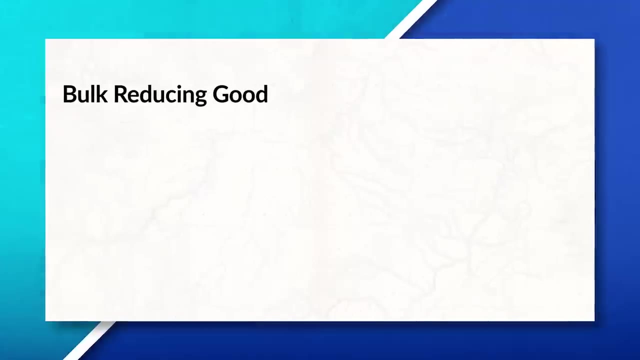 Now, before we know exactly where we should have our production be located, we have to determine if our product is a bulk-reducing good or a bulk-gaining good. Bulk-reducing goods are products that become lighter and easier to transport as they are produced. 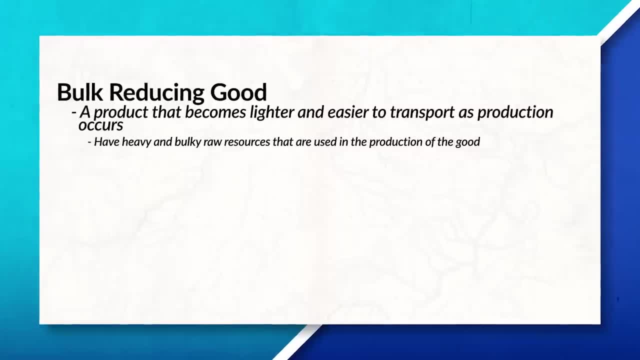 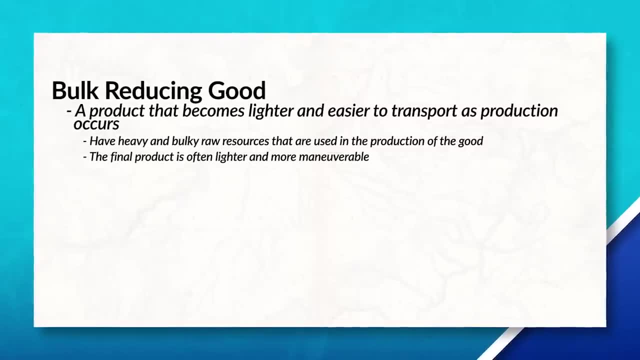 These goods have heavy and bulky raw resources that are used in the production of the good, But while the resources that are used in the production are bulky and heavy, the final product is often lighter and more maneuverable, Hence why these are known as bulk-reducing goods. 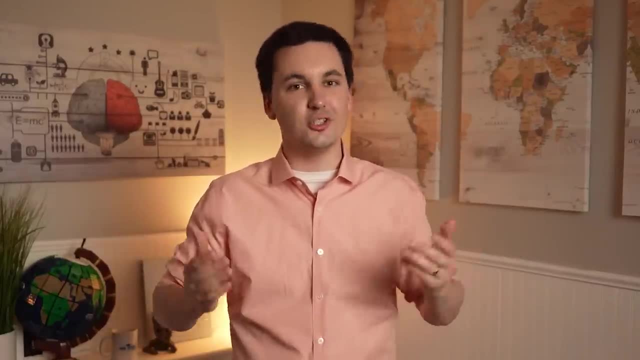 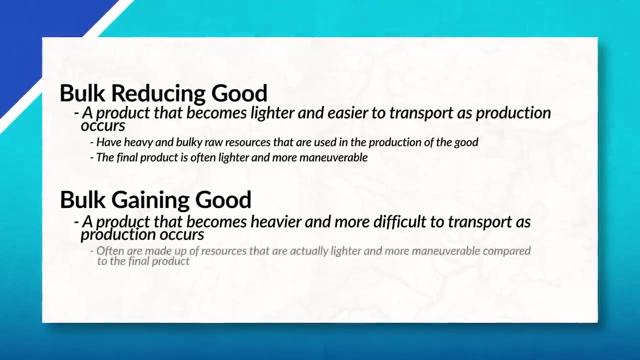 As production happens, the weight and bulk of the product reduces. On the other hand, bulk-gaining goods are products that get heavier and more difficult to transport as the production occurs. These goods are often made up of resources that are actually lighter and more maneuverable. 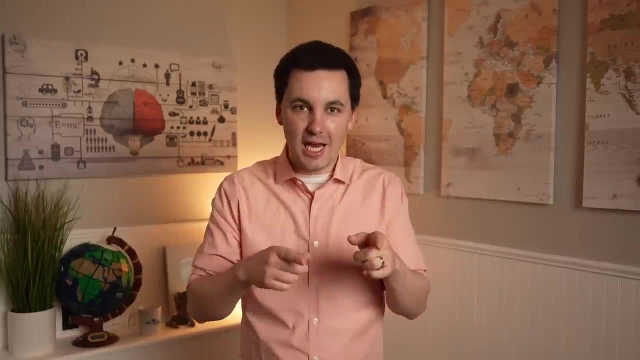 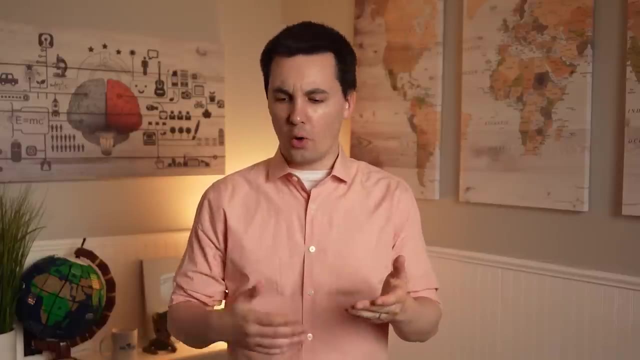 compared to the final product. Hence why these are known as bulk-gaining goods. As production happens, the weight and bulk of the product increases. Understanding if a good is bulk-gaining or bulk-reducing allows us to better determine where the production of a good should occur. 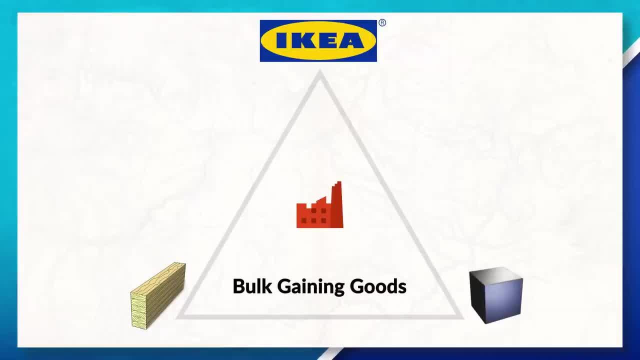 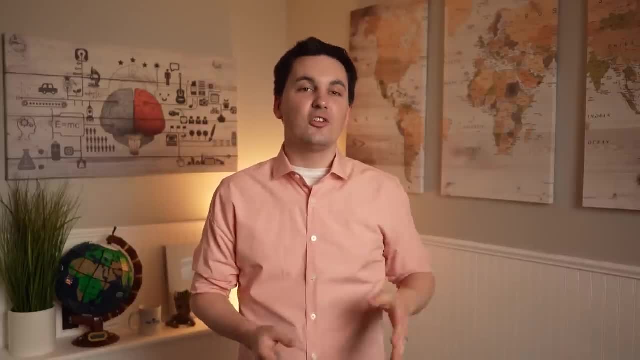 When, using Weber's theory, we can see that bulk-gaining goods are more likely to have their production be closer to the market. This ends up decreasing the amount of money that the company spends on shipping, since now they won't have to ship the heavier final product as far. 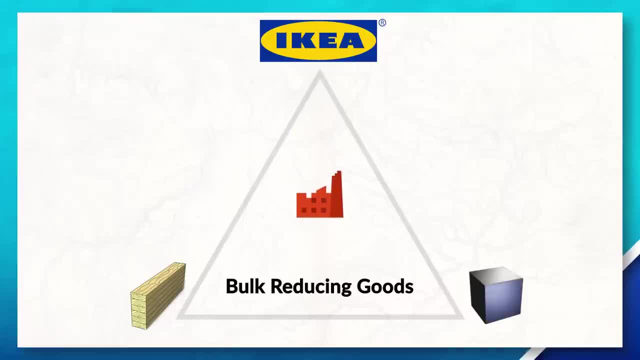 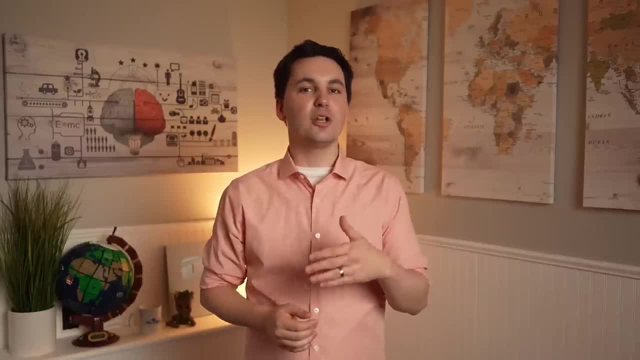 While, on the other hand, goods that are bulk-reducing are more likely to have their production be located near the raw resources instead of near the market. This is because it's cheaper to ship the final product farther distances than it is to ship the raw resources. 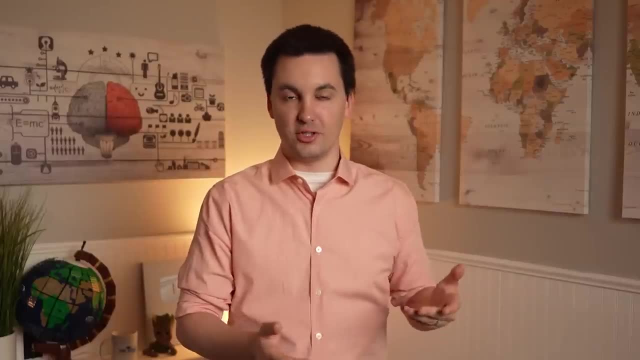 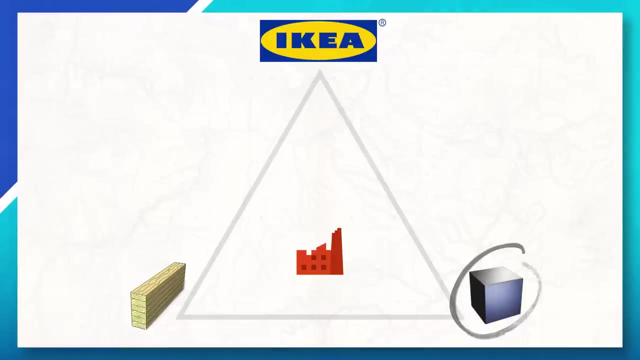 that are used to make the product. Now, just because a good is bulk-reducing doesn't mean we'll locate our production facility in the middle of the two resources If one of the resources is heavier and bulkier than the other one. 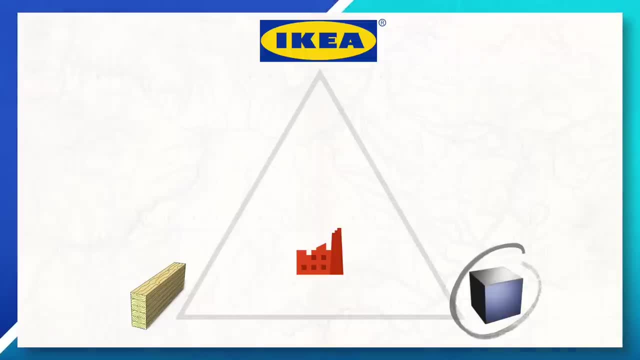 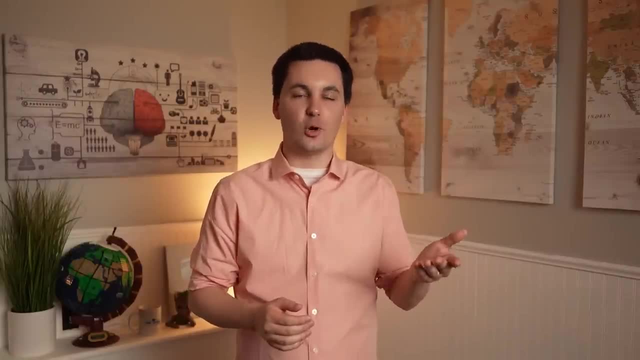 meaning that it'd be more expensive to transport. it's more likely that the facility will be located near the heavier and bulkier resource. This is because it's in the company's best interest to locate near the resource that is heavier to transport. That way, it reduces the amount of transportation. 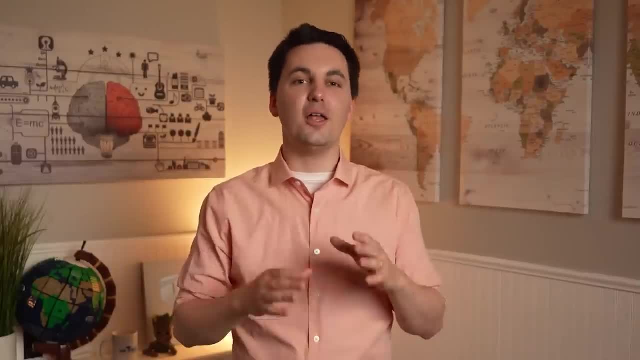 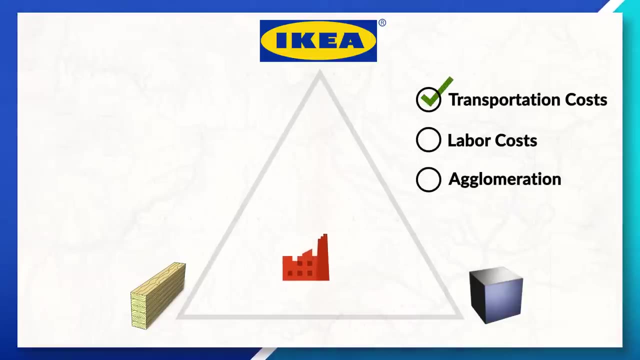 needed for that resource, all of which helps reduce the cost of production and minimize the transportation costs that the company has. So we can see that by using Weber's Lease Cost Theory, companies can reduce their overall costs and maximize their profit, all by locating in an area. 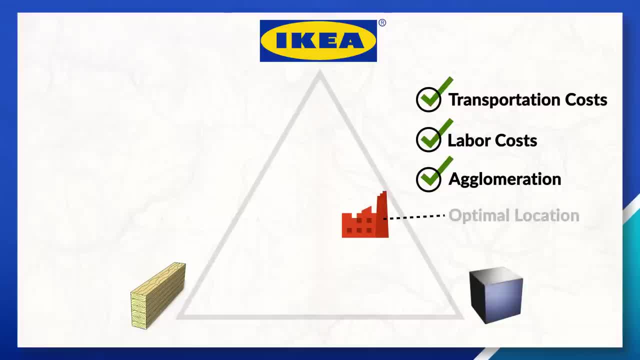 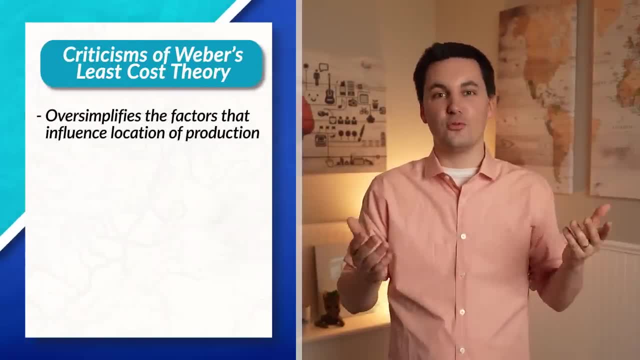 that optimizes their transportation costs, labor costs and the benefits they get from agglomeration. Now today, Weber's Lease Cost Theory has been criticized for oversimplifying the different factors that influence the location, the location of production. It also fails to consider other factors.